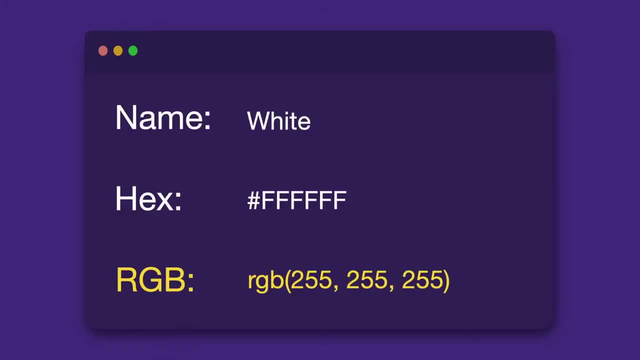 And finally, we have the RGB values, which stands for red, green and blue. So, as you'd expect, it's made up of three sets of numbers: one for red, one for green and one for blue. These numbers range from 0 to 255. 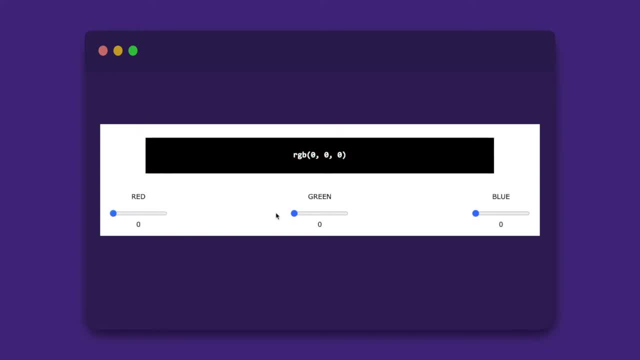 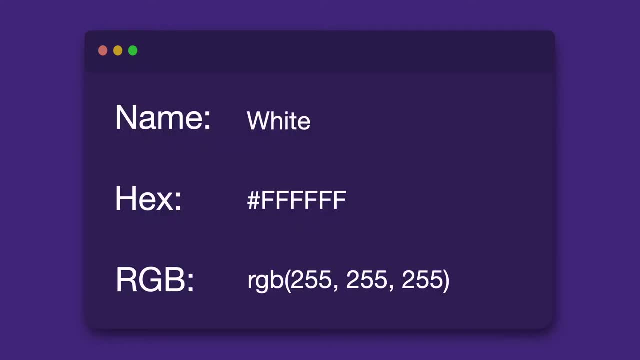 And in the same way as the hex codes. as you adjust each set of numbers, you'll create different colours. So these are the three main ways you can apply colours in CSS. Which one you use is up to you. You might be wondering: how should I know which numbers make up each colour? 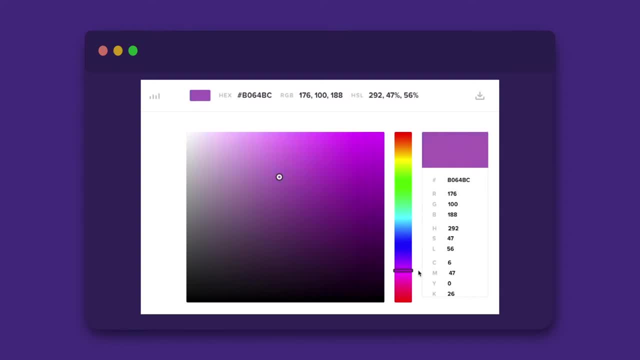 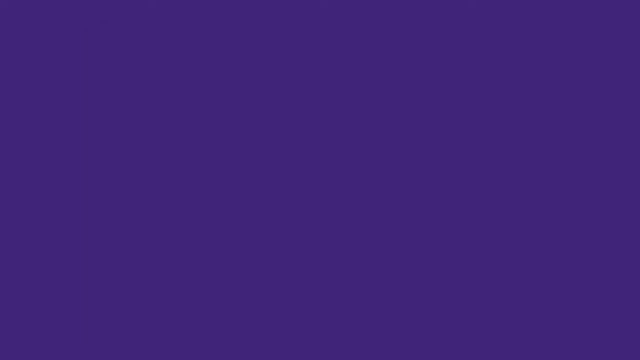 Well, luckily, there's lots of websites out there, like htmlcolourcodescom, where they allow you to pick your colour and it gives you the relevant hex code or RGB value. So now let's apply some colour to our webpage. First, let's open our text editor. 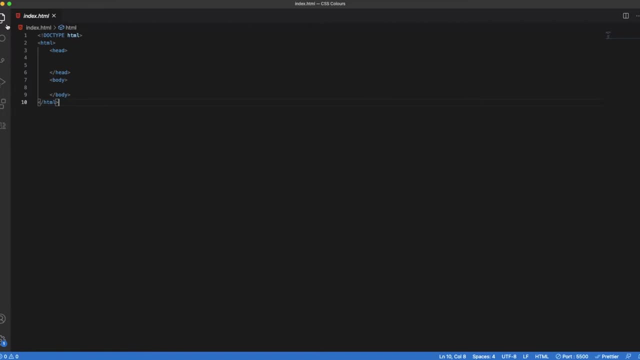 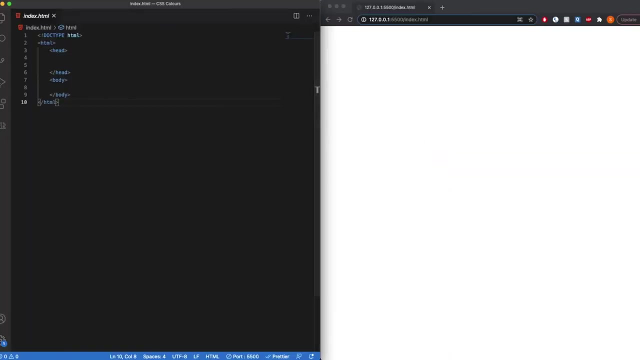 And then open a copy of the HTML boilerplate that we should be used to using by now. We can then set up the webpage so it's next to our code editor, And that way we can see what we're building as we code. So let's add a title in the header and we'll call it colours. 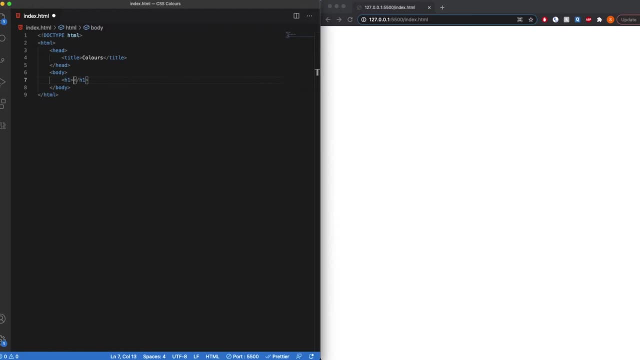 And then, if we go to the body, we can add a h1 tag for the page title And add let's learn about colours. We can then add a subheader saying ways to apply colour And we can finally add a paragraph saying let's apply some colour. 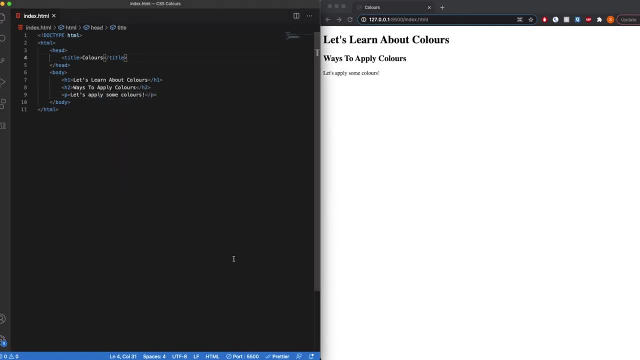 Next, we can set up our style sheet. We're going to use an internal one for this, But the same concepts apply whether you're using inline or external CSS as well. So let's add our style tag in the head element and that sets up our internal style sheet. 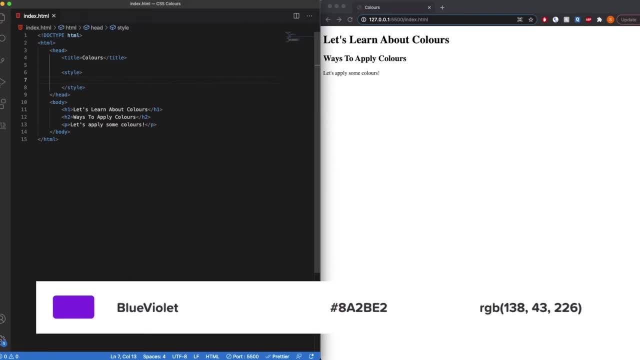 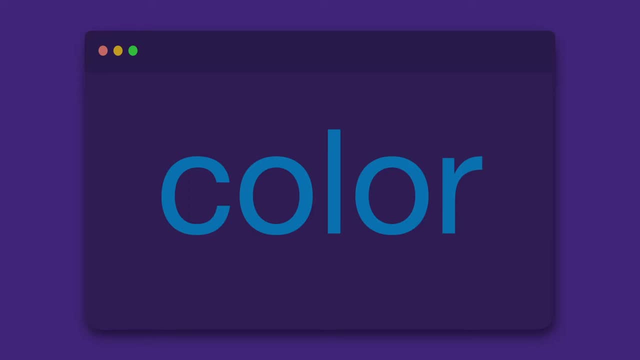 So first let's change the text colour for all three elements to blue violet. So to change the colour of the text we can use a CSS property called colour, And remember it needs to be followed by a colon, And then you can add the value. 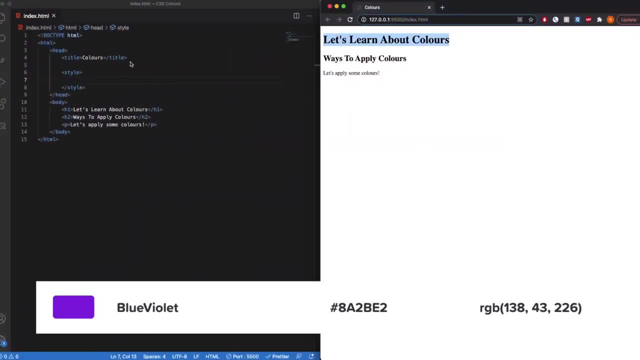 So first let's change the colour of our h1 title. We can use the h1 selector and open our curly braces, And then we can write our declaration, So we can declare the property colour, followed by a colon, And then add the value- blue, violet- followed by a semicolon. 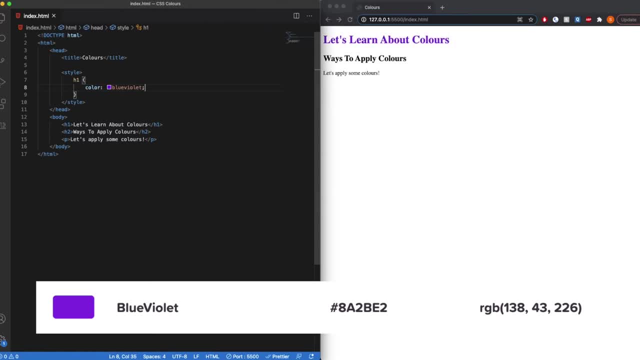 And now, if we hit save and refresh, we have our violet header. Let's do the same with the h2 tag, But this time let's use the hex code instead, So we can write our h2 selector with the curly braces. 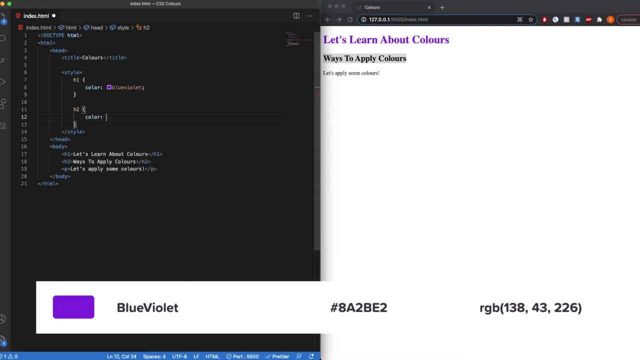 declare our property of colour and apply our hex code of 8a, 2b, e2.. So you can see both headers are the same colour. It doesn't matter whether we use the colour name or the hex code. So you can probably guess what we're going to do with the paragraph. 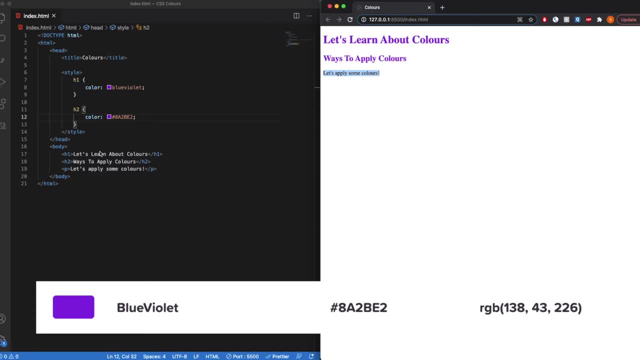 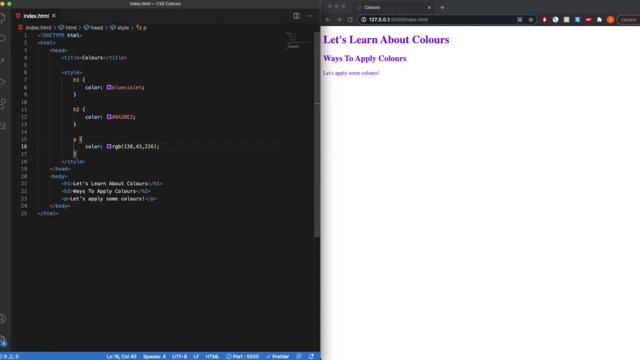 Let's apply the same blue violet colour, but using the RGB values. You should be a pro at this by now. So let's use our paragraph selector, open our curly braces and then apply the RGB value to the colour property, But say for the paragraph: we actually wanted to adjust the colour slightly. 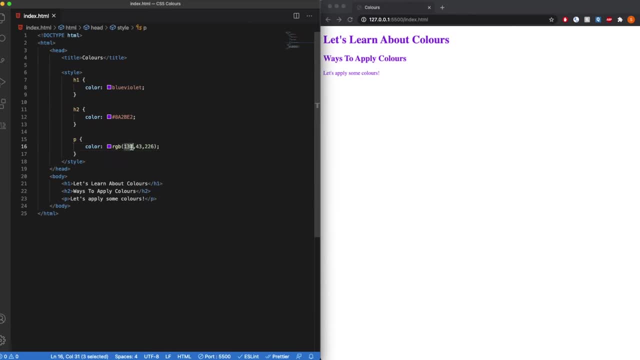 We can then change the value. so let's increase red to 255.. And now you can see the text is more pink, And this is why the ability to be more specific with hex codes and RGB values comes in handy. You can create any colour that you want. 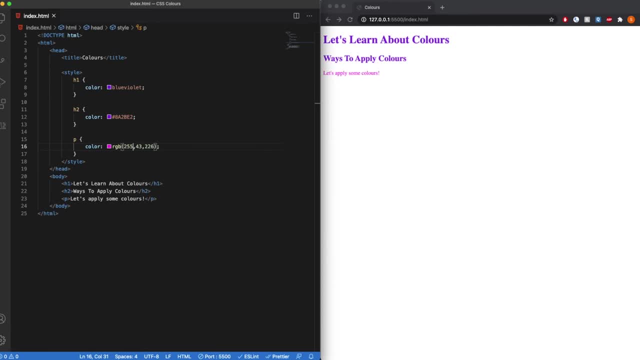 However, sometimes you might have a name colour that you like and want to use, and that's perfectly fine too. You can apply colours to lots of elements. You can change the text colour, like we've done here, or you can change the colours of borders or backgrounds. 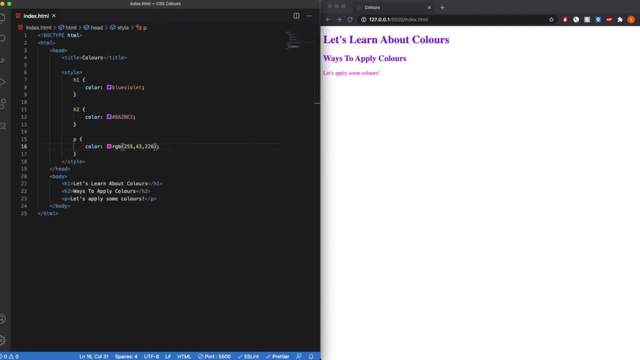 and we'll be covering these in the next few videos. And when developing websites, it's important to make them accessible for people who are colour blind as well, So keep an eye out, as we'll be releasing more videos on this shortly. Hopefully, this gives you a good introduction to how colours are made on the web. 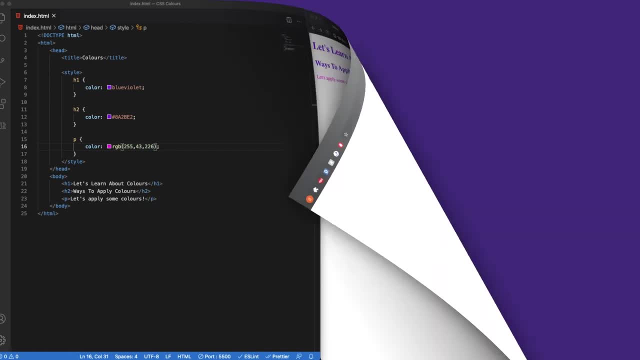 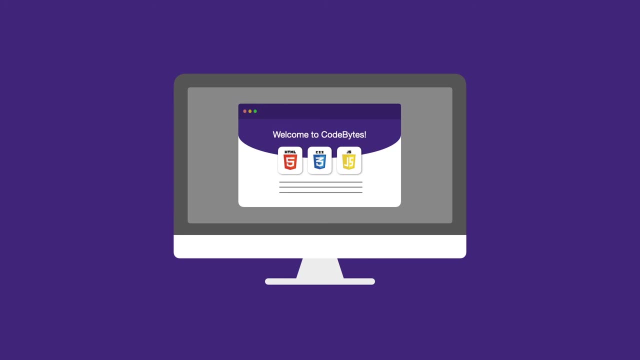 and how you can create and apply any colours that you like to your webpage. You can find all the code from our tutorials on our website or GitHub page, And remember that when following tutorials, don't just copy and paste the code, but make sure you take the time to understand the concepts. 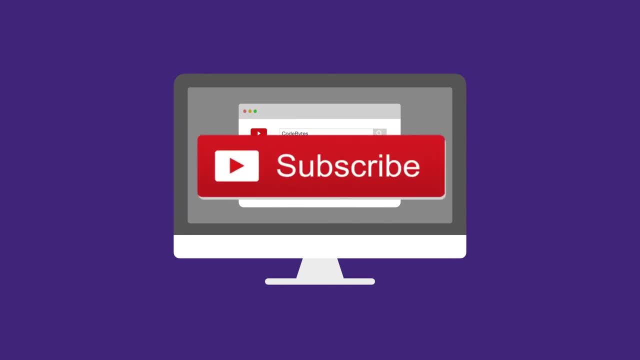 If you want to see more videos like this, hit the subscribe button below. We'll be releasing new content weekly and, in the meantime, for more web development inspiration and advice, you can follow our social media accounts, which are linked in the description below.